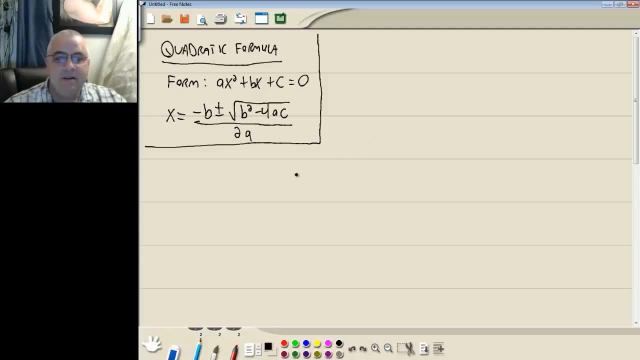 Let's take a look at a problem. The first one here has 21x squared plus x minus two is equal to zero. 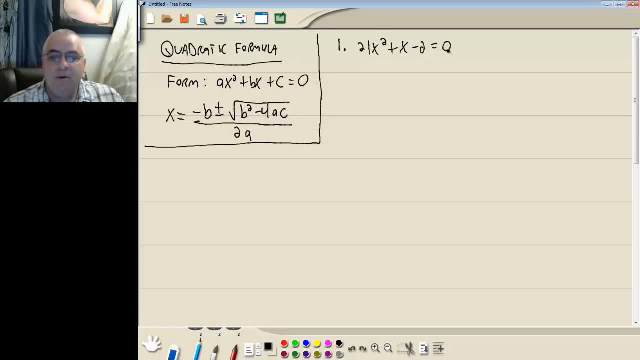 It says you can solve by using the quadratic formula. It's in right form as we have zero on this side, and it's a quadratic. So the first thing to do is identify our a, b and c. 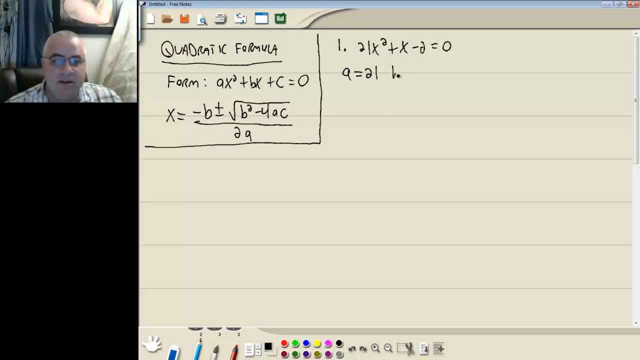 a is whatever number is in front of your squared which is twenty-one. b is whatever numbers in front of your x, which is 1, and c is your number at the end, which is a negative 2. Now, unless you don't mess up on signs, it's a good idea to go through and replace all of your variables with sets of parentheses before you plug in your numbers. So we're going to have x is equal to negative b plus or minus square root of b squared minus 4 times a times c all over 2a. And now we'll plug in where we identified. We said a was 21, so everywhere we had an a, we'll put in 21. We said b was 1, so everywhere we have a b, we'll put in 1. And we said c was negative 2, so everywhere we have a c, we'll put in negative 2. And now you want to simplify. So we've got negative 1 plus or minus square root. 1 squared is 1. Negative 4 times 21 gives us 84 times, well, negative times positive is negative times another negative is positive. So 84 times 2 gives us 168. So we've got 1 plus 168 over 2 times 21 is 42. So we've got 1 plus 168 over 2 times 21 is 42. So we've got 1 plus 168 over 2 times 21 is 42. 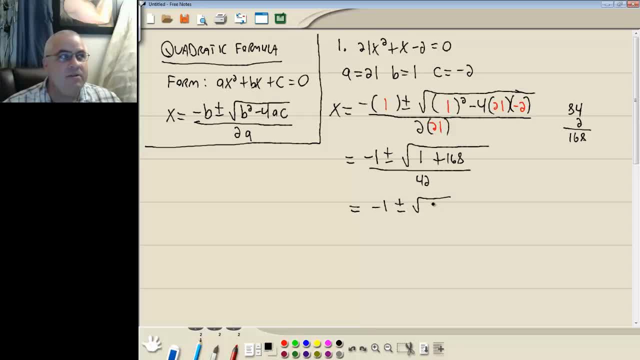 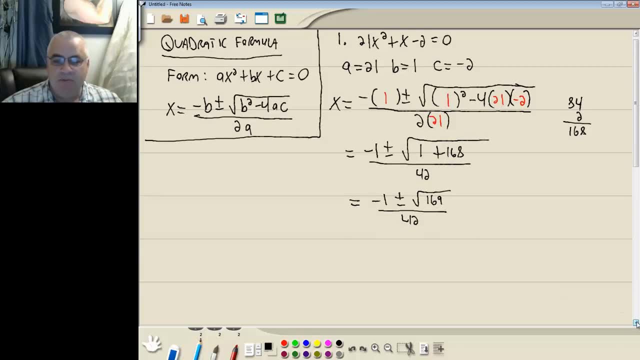 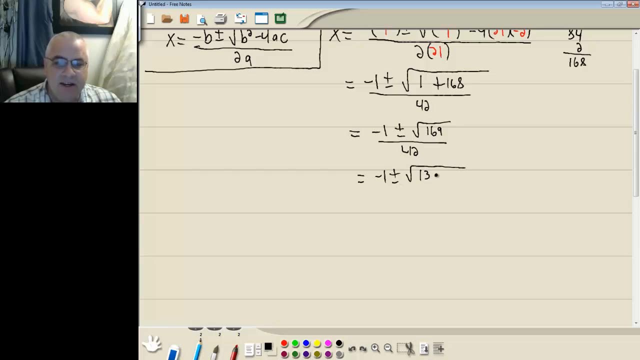 So we've got negative 1 plus or minus. 1 plus 168 is 169, all over 42. And you should always simplify your radicals before you go on. 169, that's 13 times 13. Remember with square roots, we're looking for pairs or something. So here's a pair of 13s. A pair of 13s is going to come out in front as a single 13. 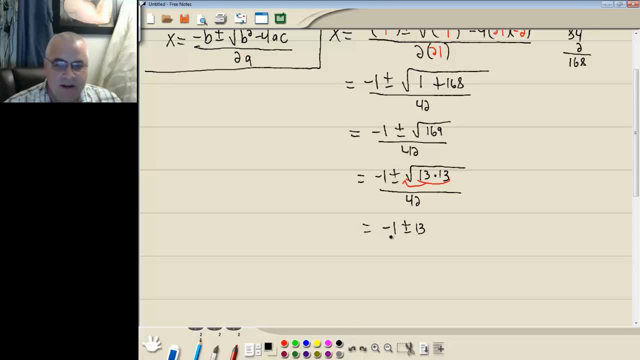 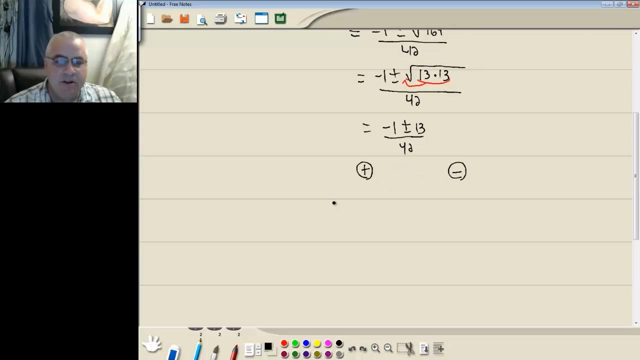 So we've got negative 1 plus or minus 13 over 42. Now if your radical disappears, then it's a good idea for you to split them up into two separate pieces. We're going to have a positive version, we'll have a negative version. What that plus or minus means is we'll have negative 1 plus 13 over 42, and we'll have negative 1 minus 13 over 42. And again, if 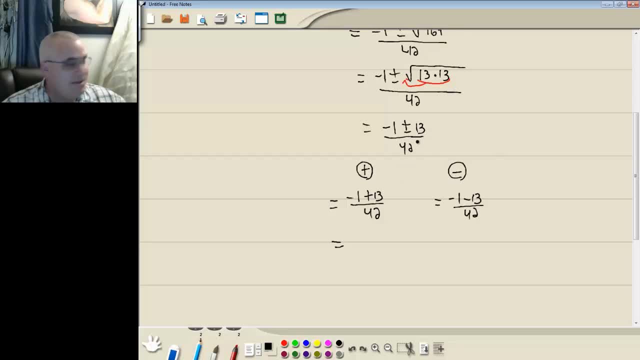 your partial셩 colonizeval, you'll have something like 34oker. So you can slip that into this. ahora sin арima sin. 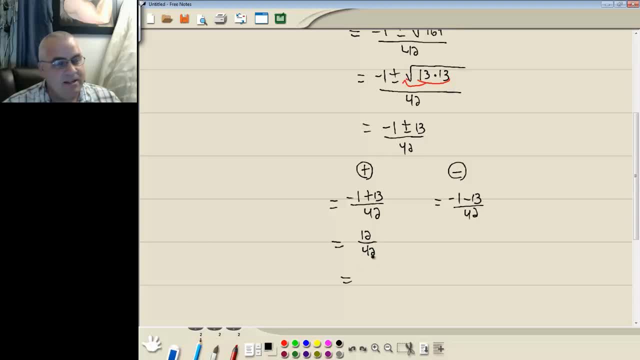 Well, negative 1 plus 13 is 12. All over 42. That simplifies- 12 and 42 both for visit to 6. 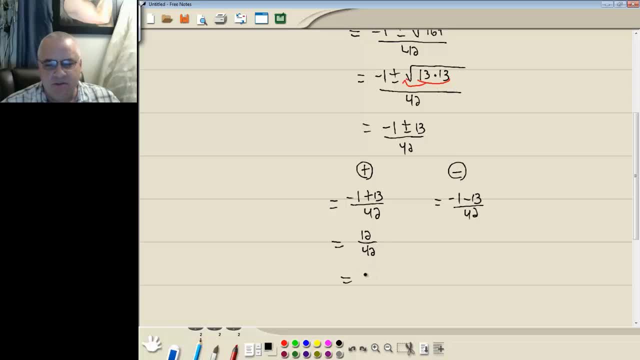 12 1 plus 3 is 1 plus 6 is 12. So that gives us two sevens. Now you can change that. Negative one negative 13 is negative 14 42. 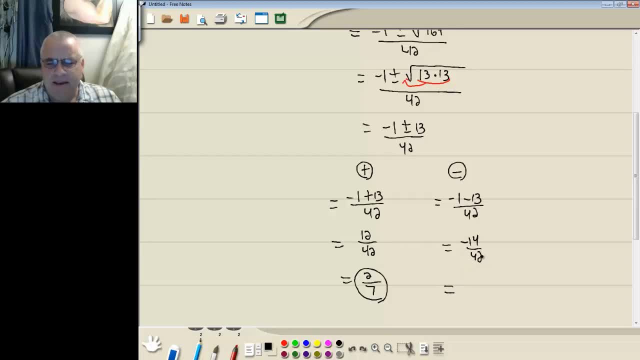 42 and I believe these are both divisible by 14 just from past semesters typically I just see the 7 but I think it's more than that but let's do the 7 just because I'm not sure negative 14 divided by 7 is negative 2 42 divided by 7 is 6 and I see it does reduce some more so that gives us negative 1 3rd so those would be your two answers for that problem yeah start new page 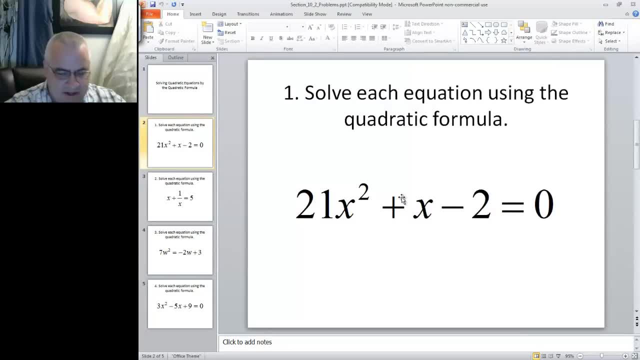 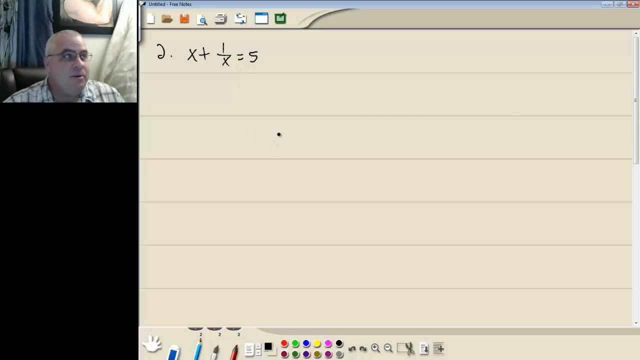 here let's look at our second example so we got X plus 1 over X is equal to 5 this is not in the right form it's not a quadratic we don't have an x squared well if we think about our test for solving any kind of equation almost our first step we do is get rid of fractions and you do that always the same way you multiply everything by the LCM of all your denominators now we only 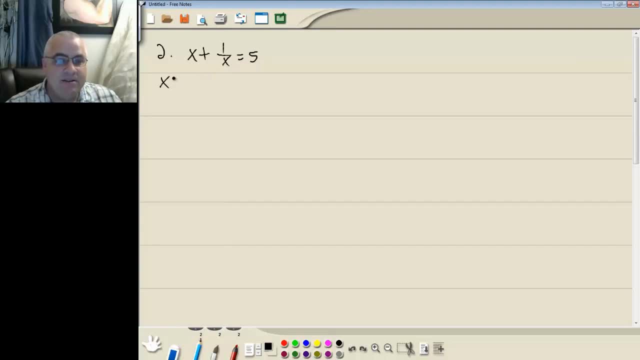 have one denominator the X so we're gonna multiply everything by X so take x times X I'll take X times 1 over X and x times 5 x times X is x squared those X's cancel so we got plus 1 equals 5 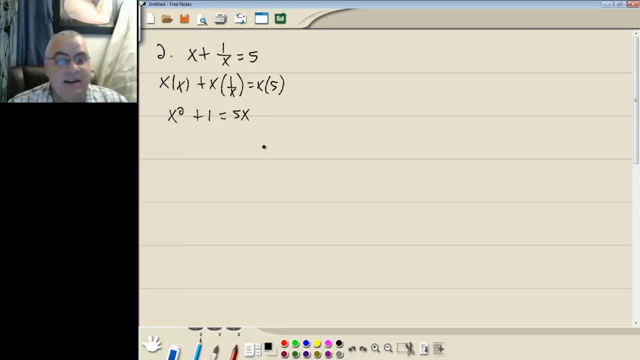 5x. Now this is starting to look closer. This is um looks like quadratic. So let's get everything over one side zero on the other. So I'll take 5x to the left side and we got x squared minus 5x plus 1 equal to 0. And now it's in the right form. It's quadratic and we got zero on one side. 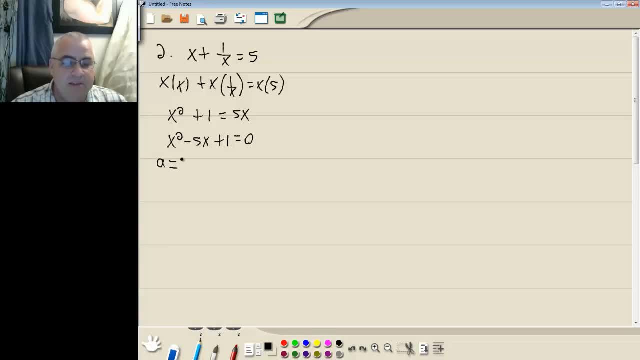 Let's identify our a, b, and c. A is whatever numbers in front of your x squared which is 1. B is whatever numbers in front of your x which is negative 5. And c is your number at the end which is 1. Our quadratic formula. We're going to have negative b plus or minus square root of b squared minus 4 times a times c all over 2a. And put little letters underneath there. Negative b plus or minus b squared. 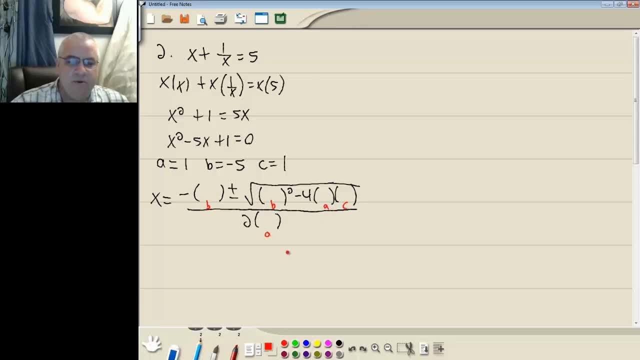 Minus 4ac all over 2a. Okay we said a was 1. So wherever we had an a we'll put in 1. We said b was negative 5. So wherever we have b we'll put in negative 5. And we said c was 1. So wherever we have a c we'll put in 1. Well negative negative gives us a positive 5 plus or minus. Negative 5 squared is 25 minus 4 times 1 times 1 is 4 all over 2. Which gives us 5 plus or minus 25 minus 4 is 21 over 2. And that's our answer. Now we don't try to split this up into a positive version negative version because the radical didn't disappear. So it wouldn't benefit us to split it up. Sometimes you'll split it up because you have an imaginary part. But that's okay. You can split it up because you have an imaginary part. But that's okay. You can split it up because you have an imaginary part. But that's 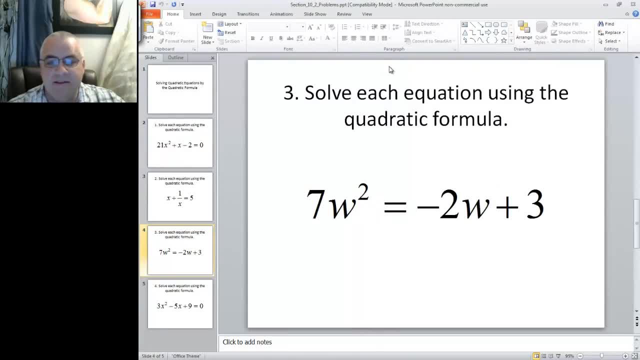 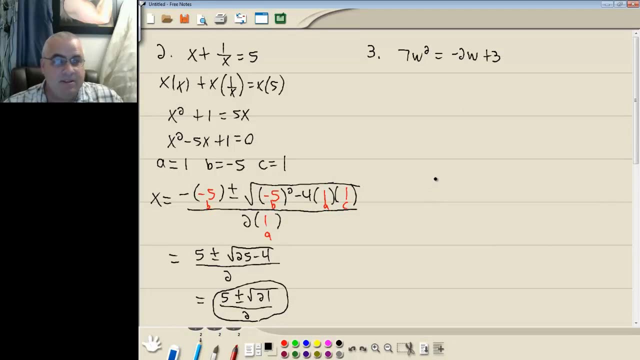 a different different case. Let's take a look at this one. So we've got 7w squared is equal to negative 2w plus 3. Now this is a quadratic. It's a different variable. It's not x but same idea. This is a quadratic. So we don't get everything over one side zero on the other. So I'm going to have 7w squared take negative 2w over becomes a positive 2w. 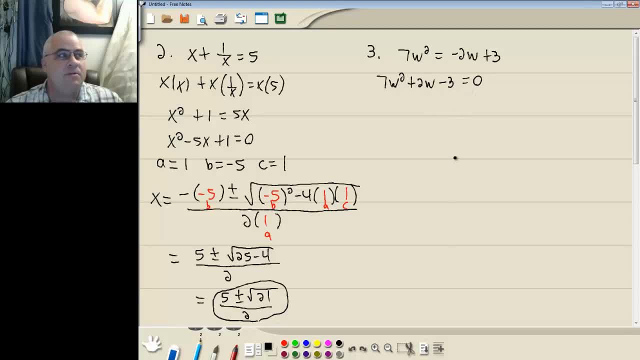 Take 3 over becomes a negative 3 equals zero. Again it's quadratic. We get zero on one side. So now we can start with our formula. A is whatever is in front of your w squared which is 7. B is whatever is in front of your w which is 2. And C is your number at the end which is negative 3. Our formula says x equals negative b plus or minus square root b squared. Minus 4 times a times c all over 2a. Label that. That's b and this is b, a, c all over 2a. Okay we said a was 7. So everywhere we had an a we'll put in 7. Said b was 2. So everywhere we had b we'll put in 2. And c was negative 3. 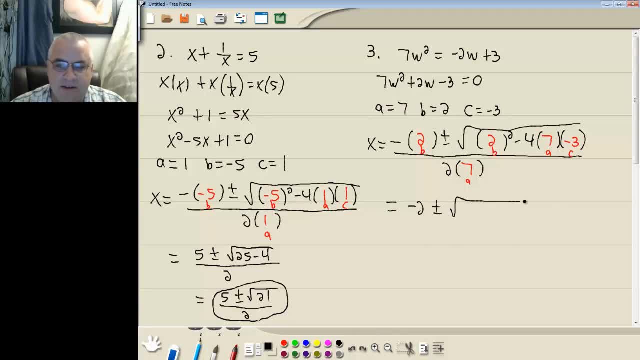 So I got negative 2 plus or minus. 2 squared is 4. Negative 4 times 7 is negative 28 times a negative 3. I don't know what it is yet but it's positive. 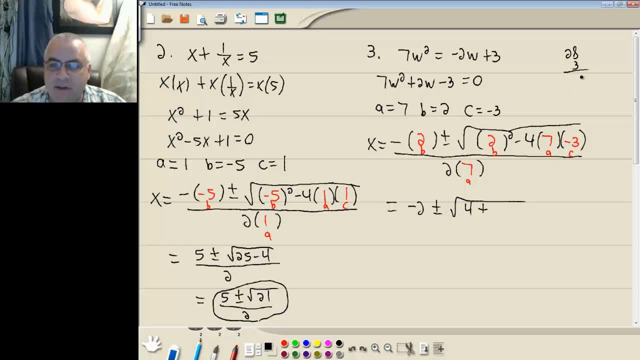 4 times 7 is 28 times 3. 84. Over 14. Okay so that gives us negative 2 plus or minus. Square root of. 2. Minus. 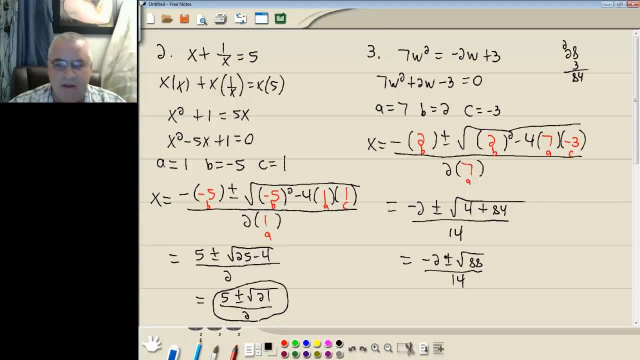 Of 88 over 14. Now always you should simplify a radical before you go on. 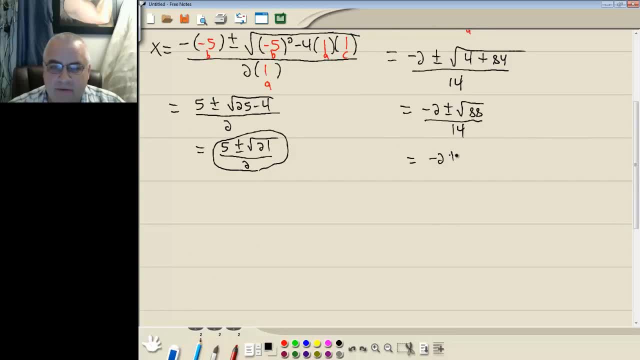 And that's what we'll do here. So we got negative 2 plus or minus. Square root 88. 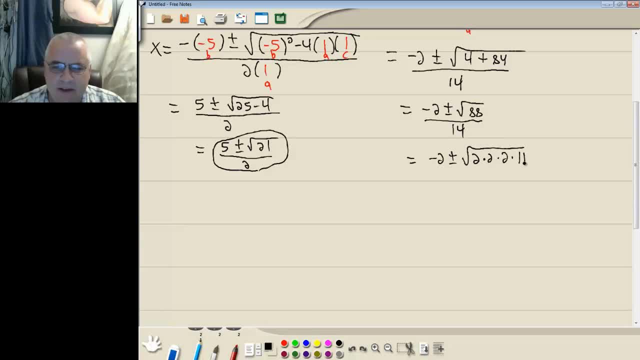 That's 2, 4, 8 times 11. All over 14. Now remember we're looking for pairs of something. Here's a pair of 2's. 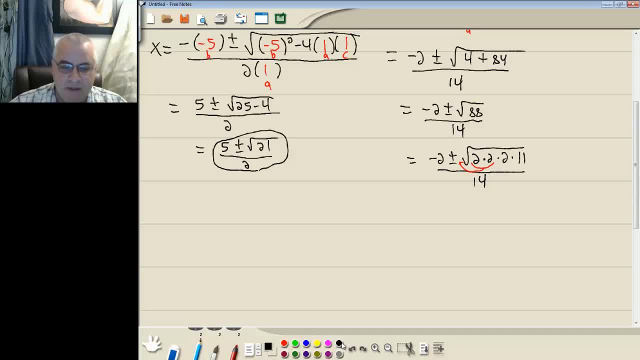 So those pair of 2's are going to come out in front as a single 2. So we got negative 2 plus or minus 2 square root and we're left with a 2 and 11 inside. And you can only bring something out if it's a pair. 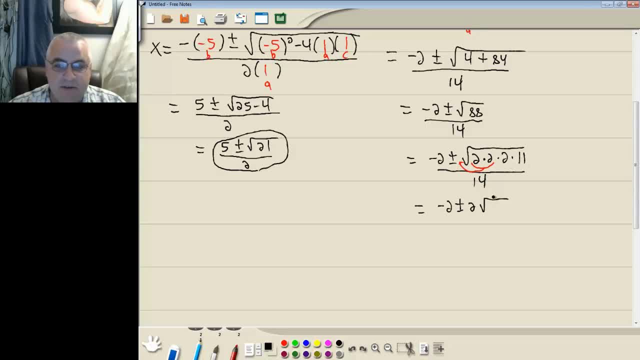 We don't got a pair of 2's or 11's so we just multiply these together. 2 times 11 is 22 over 14. 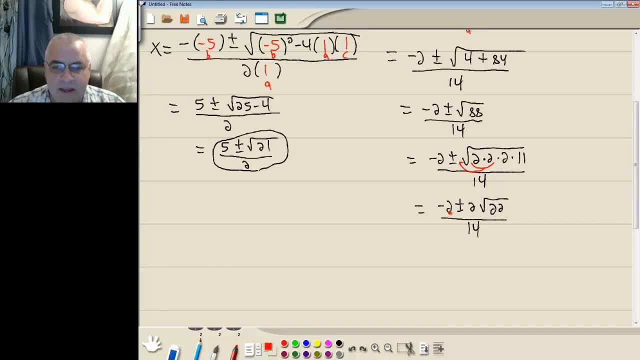 Now this is something that pops up fairly often in the quadratic formula. If you can divide this number, this number, and this number by the same number do so. And those are all divisible by 2. 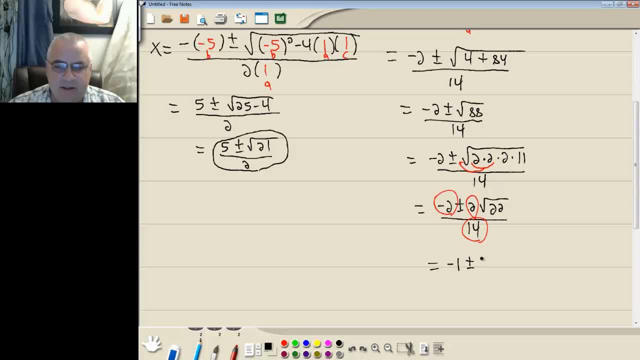 So we're going to get negative 1 plus or minus 1 square root of 22 over 7. 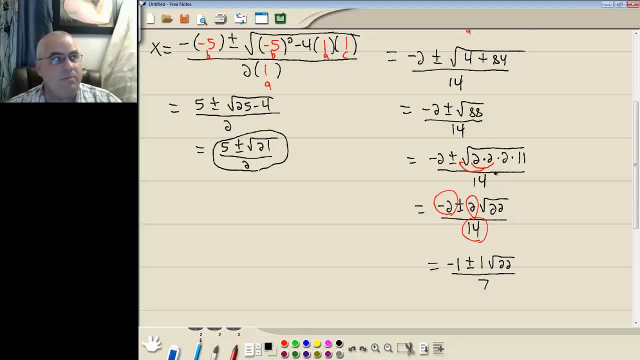 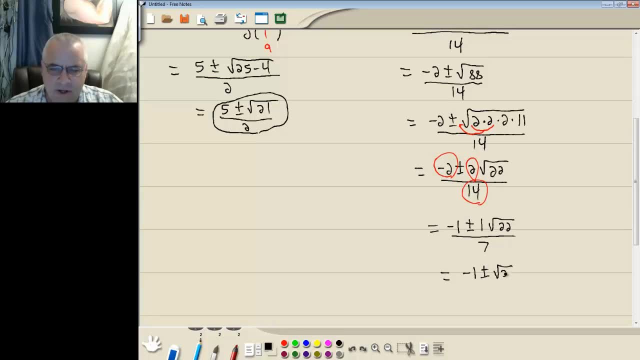 Now notice I do not touch what's inside the radical at all. I just touch those three numbers. So that's going to give us negative 1 plus or minus square root of 22 over 7. 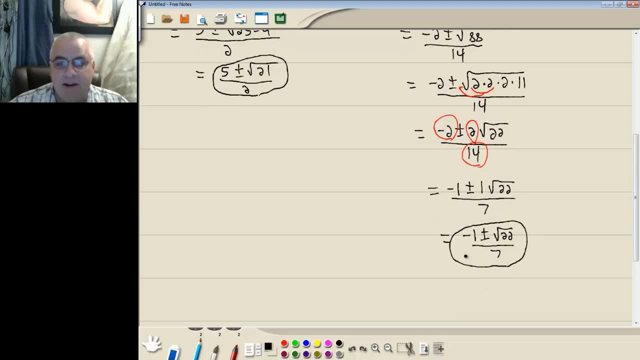 Again I do not split that up into two separate pieces because the radical didn't disappear. 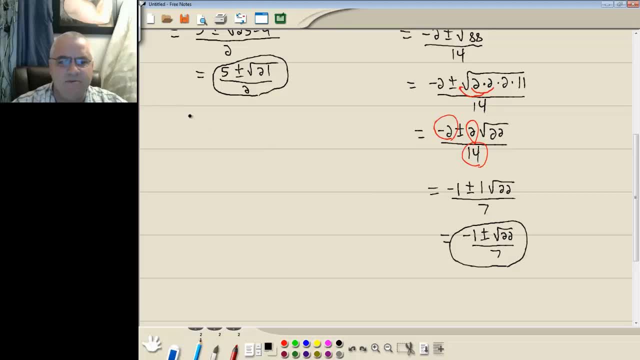 Let's take a look at this one. We got 3x squared minus 5x plus 9 equal to 0. It's already a quadratic. It has 0 on one side so it's already in the right form. So let's just signify our a, b, and c. 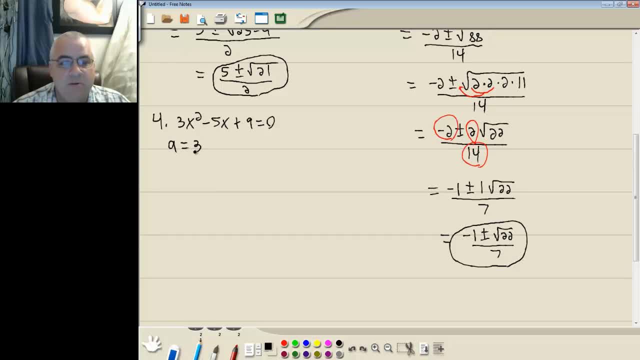 a is whatever number is in front of your x squared which is 3. b is whatever number is in front of your x which is negative 5. And c is your number at the end which is 9. 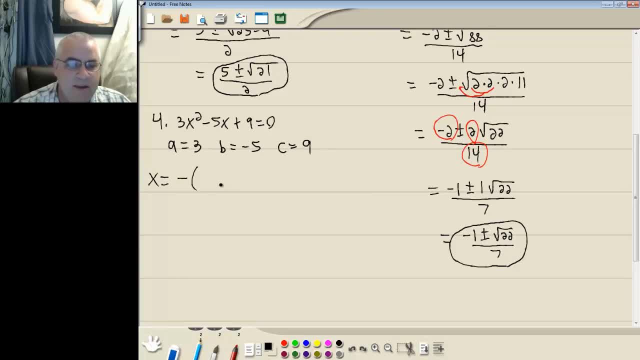 So we're going to have x is equal to negative b plus or minus square root of b squared minus 4 times a times c all over 2a. 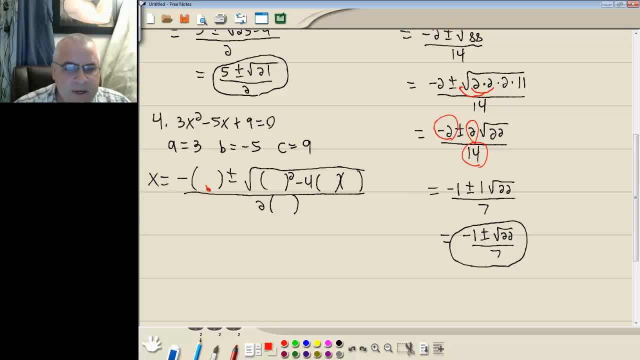 I'm going to label these. This is b, b, a, c, and a. Okay, we said a was 3 so everywhere we had an a we'll put in 3. We said b was negative 5. 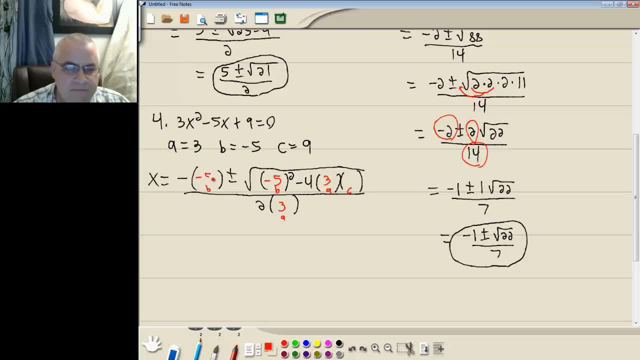 So everywhere we had a b we'll put in negative 5 and we said c was 9 so everywhere we had a c we'll put in 9. 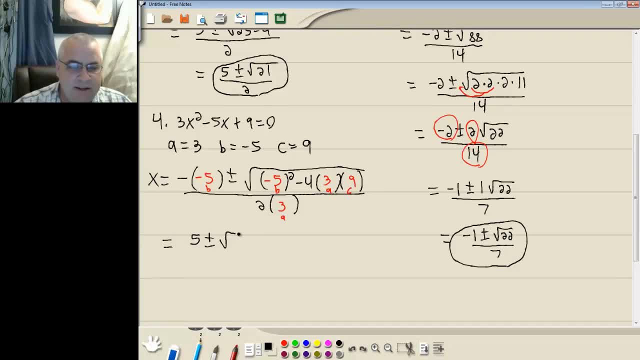 Negative negative gives us a positive so we got positive 5 plus or minus square root negative 5 squared is 25 minus 4 times 3 is 12 times 9 gives us 108.